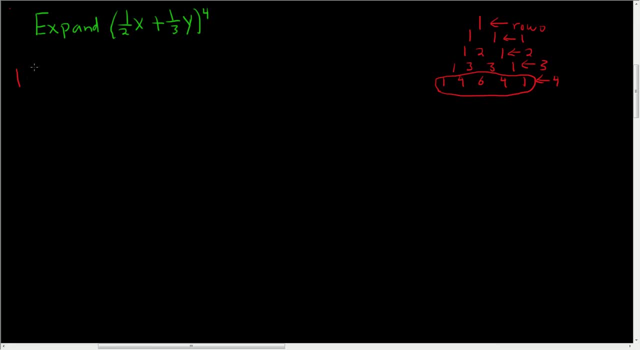 So 1.. And then we'll write the first term, so 1 half x, And we always start with this number here. So this is a 4,, so you put a 4.. Then you write the next one, 1, third y, And we write a 0.. 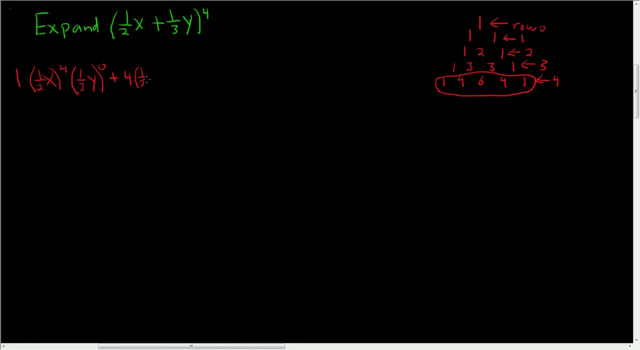 Plus 4, 1 half x. Now we go down 1.. So 4 minus 1 is 3.. 1 third y. And then you add 1 here. 0 plus 1.. 1 is 1.. Plus the next coefficient is 6.. And then 1 half x squared And then 1 third y squared. It's really easy to mess up in this next step And again you'll notice the pattern: 4, 3, 2, 0, 1, 2.. Now they're both 2, so it's easy to get mixed up. So 4, 1 half x. 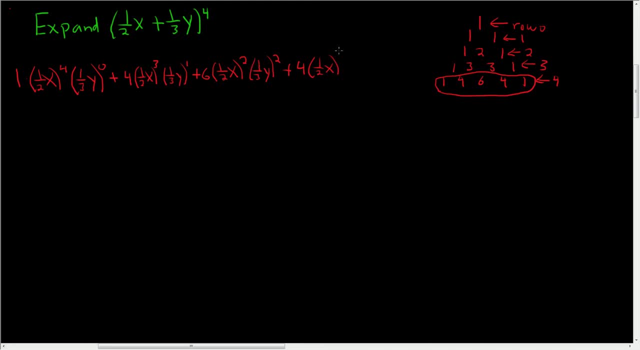 And this one is going down. So we go from 2 to 1.. 1 third y cubed, And the last one is plus 1. 1 half x to the 0. And then 1 third y to the 4th. Wow, that's really small, Okay. so let's write it up. Let's clean this up Now. it's usually better just to clean this all up in one step. So the first term: 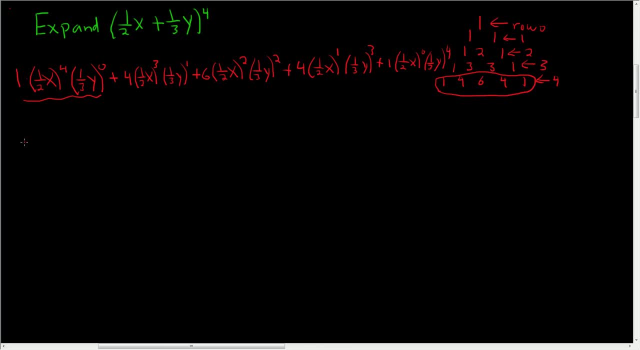 it's 1 half and it's being raised to the 4th power. So 2 to the 4th is 16.. So 1 over 16, x to the 4th, And that's 1.. Anything to the 0 power is 1.. Plus, here we're going to get a 4.. We're going to get a 1 eighth And we're going to get a 1 third. So that's 1 half, 1 half times 1 sixth. So 1 sixth x cubed y Over, here we have a 6..